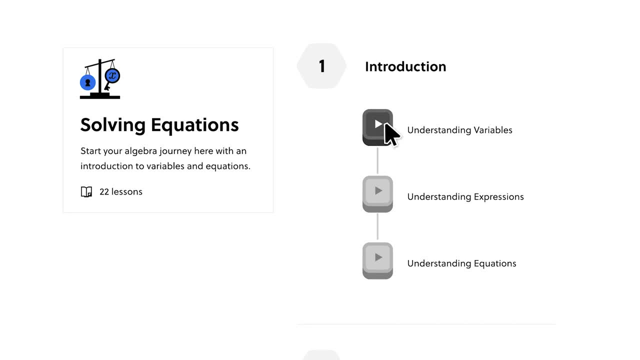 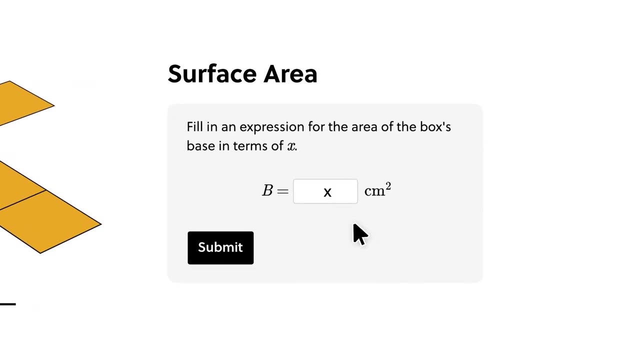 What I've loved about using Brilliant is that it just works for any age because of its interactive elements. I was checking out some maths lessons that I thought would be interesting to promote and ended up spending hours enjoying the customised lessons myself, Picking up some great new teaching tips along the way. 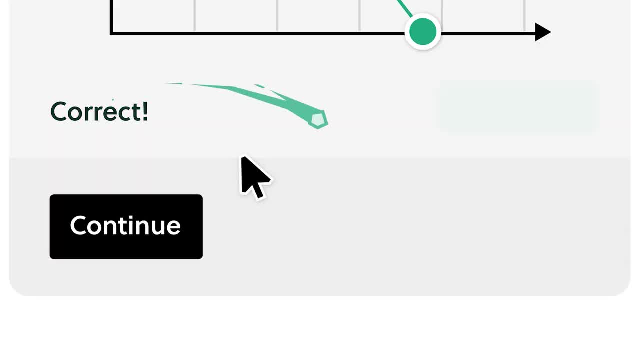 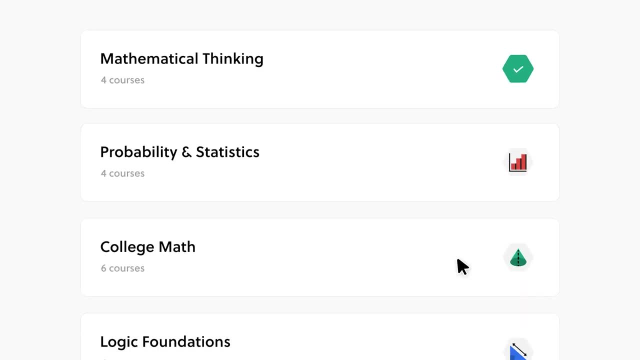 In the Solving Equations course, you aren't just told what the answer is to a problem. Brilliant provides these incredible visual representations to help you understand the concept properly. When you can move variables around through an interactive diagram, learning just becomes so much more simple. 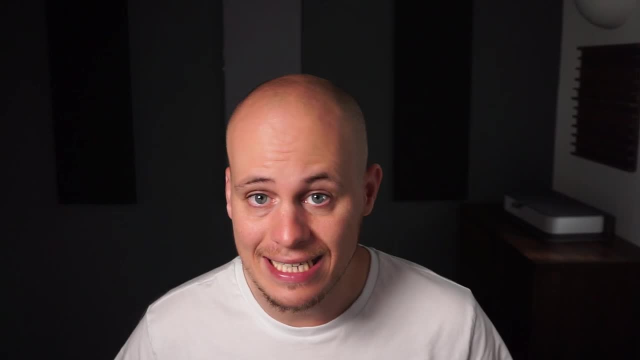 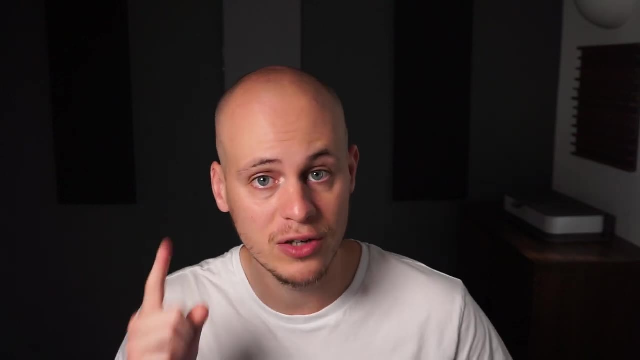 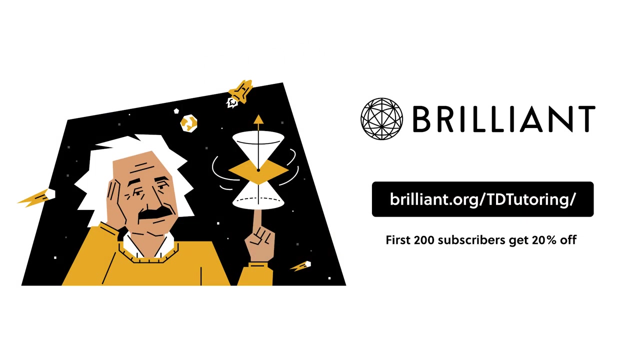 To try everything on Brilliant free for a full 30 days, simply visit wwwbrilliantorgtdtutoring, because we've managed to secure the first 200 people 20% off of their annual premium subscriptions. Oh Cubeness. 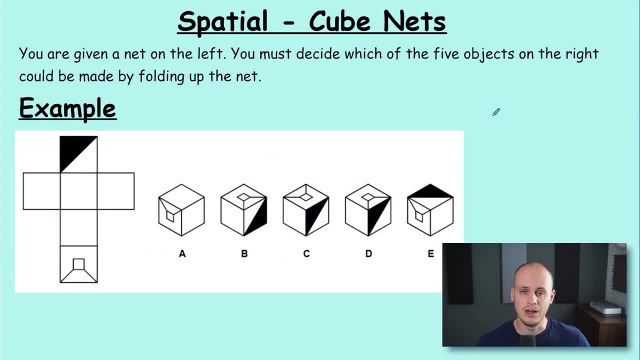 Something that we never even used to try to tackle online because it's such a tricky type of spatial reasoning. But since then we have developed some strategies and hopefully even across the screen, I can show you some ways of solving these questions a little bit more accurately each time. 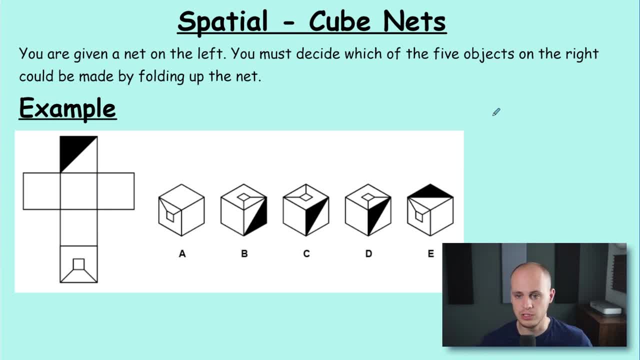 Now I will say this Parents as well: if you're listening into your children, who are watching this right now, the best thing you can do- and it will take some time with Cubeness- is actually make some of these nets in real life. 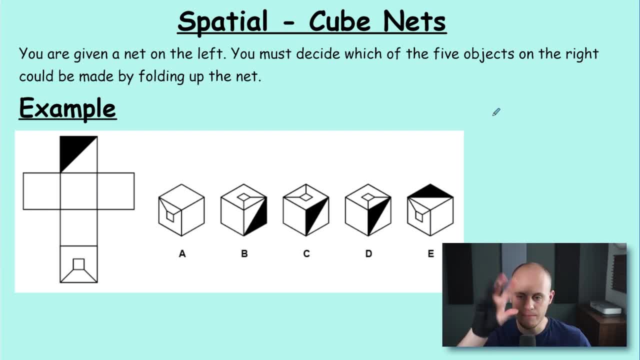 Can you draw that net? Could you use little square templates to make these nets yourself? Cut them out and fold them so that you can see and feel How they fold. The reason I find these questions easier- more easy- is because I've folded nets before. 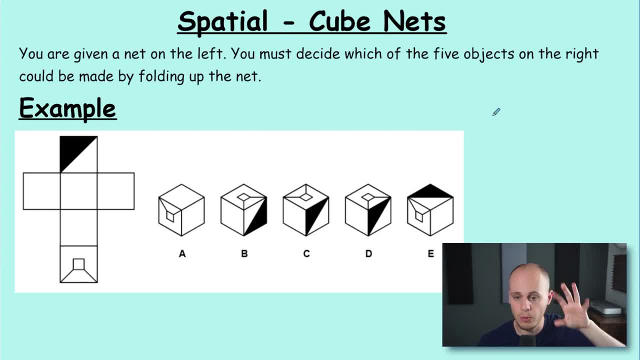 so I can imagine, I can visualize in my head what it might look like to start folding up that net Now. without that visualization, it just adds slightly, it makes it slightly more difficult. I do still have some strategies, however. that even to someone who's never folded up a net before, 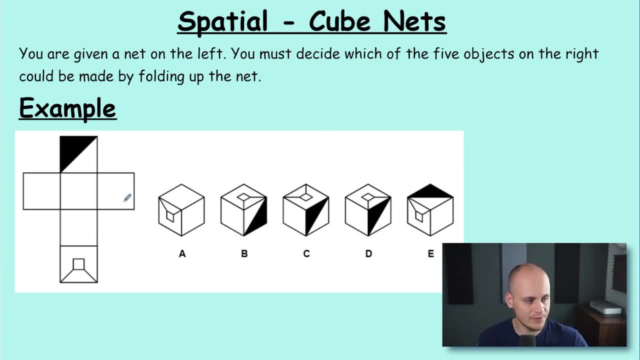 will work in solving these questions. So here's the example: You are given the net of something on the left and you simply have to pick one of the options here. that is correctly showing what it would look like if it was folded up into a cube. 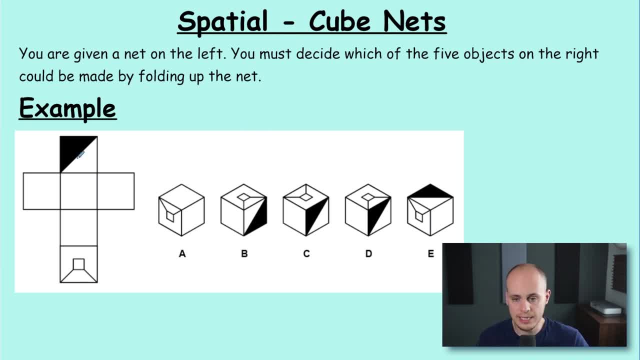 So first trick I want to show you is that the top and bottom- in fact I've got it on my next slide here- when folded, this blue side here, would meet with this blue side. okay, So you can actually represent it by taking. you could just draw the top square and draw it down here instead. 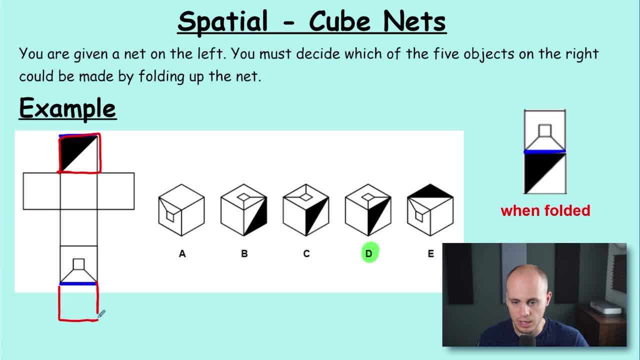 You can just alter your drawings. you know what they look like when they interact. Okay, you can just sketch it in like this: And then you know a bit more visually clear now that oh okay, so the two lines coming from that square go into the corners that meet with the face that has this black triangle on it. 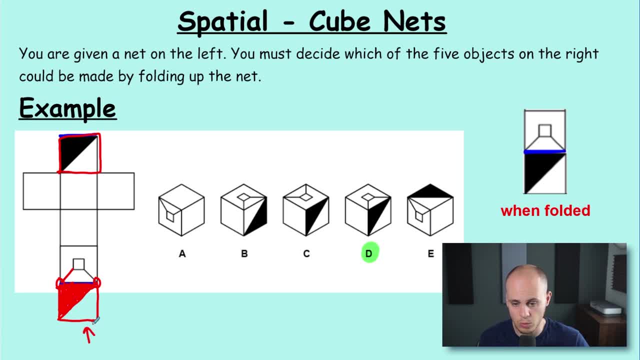 and specifically, they meet with one of the black sides, not one of the white sides of the triangle. So, for example, if you look at B, we can now get rid of B, because I've just realized that the two little lines coming from that square meet with a white side of the triangle. 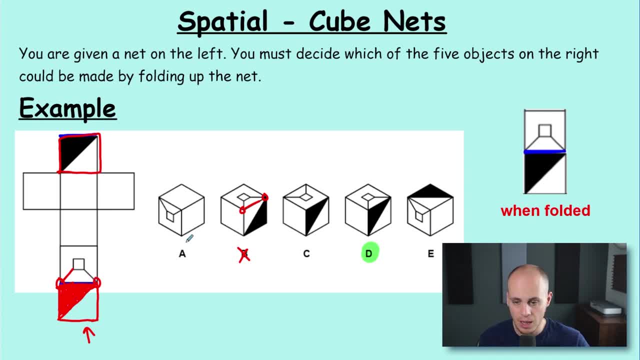 and we've quite clearly shown here that it meets with the black side. I can get rid of A as well, because it doesn't meet with anything. I can get rid of C because again the lines are going the wrong way. They're not meeting with the triangle. 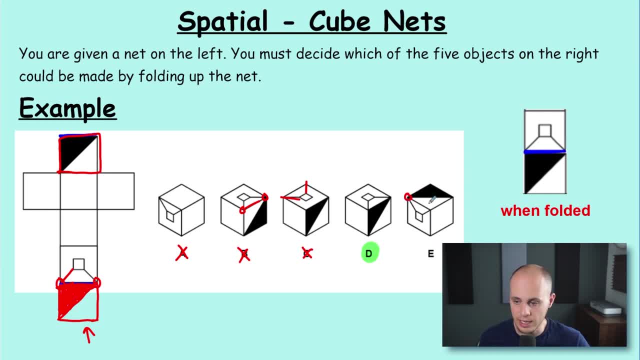 And I can get rid of E for the same reason as B. It's meeting the triangle, but it's meeting the wrong side. It's meeting the white side. D is the correct one because it fits our pattern. It meets with the black edge of the triangle. 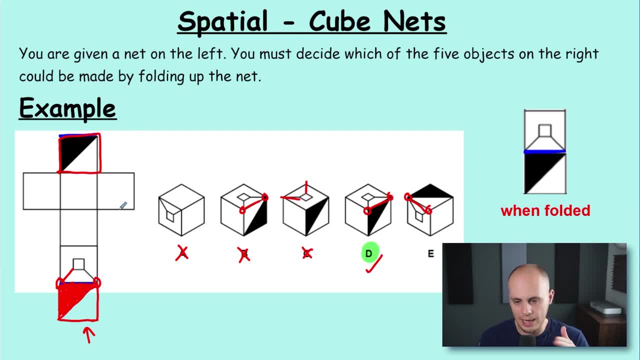 So that's the first thing you can do- is you can manipulate what the net looks like by thinking which pieces would touch. Another thing you can do- and it's really important I explain this now- is understanding opposites. So when nets are folded, if a side is two apart with one square in between them, 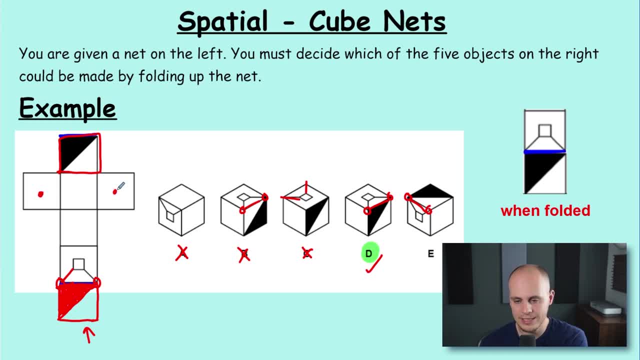 those two sides, that I've put a red dot on those two faces. they will never be next to each other, They will always be opposite. If I folded them down, they will always be perfectly opposite each other, And that works in general. 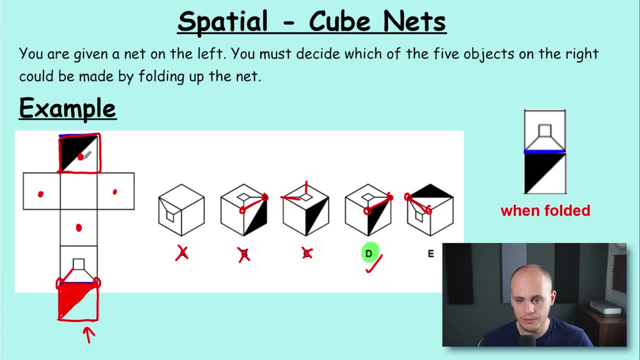 If I take this top one and I go two down now, those two ones that I've put a red dot on, they would also be opposite. And finally, I'll do it with a tick this time, that one and that one would also be opposite. 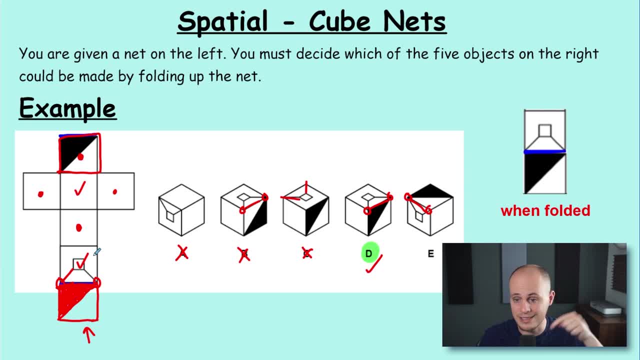 So think of that as well in twos, because you can use that to get rid of answers. If you notice that the two faces with a tick on them are next to each other in one of your answers, well then you know they're wrong, because they have to be opposite. 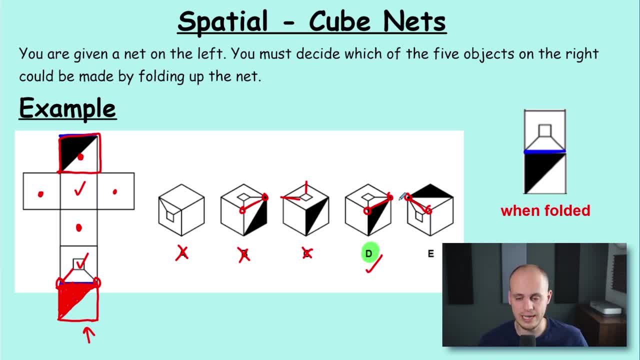 So we're going to really heavily rely on deduction today and using two or three strategies so that we know where faces are in relation to each other, and then we'll use deduction to get rid of wrong answers And we'll see how successful that is. 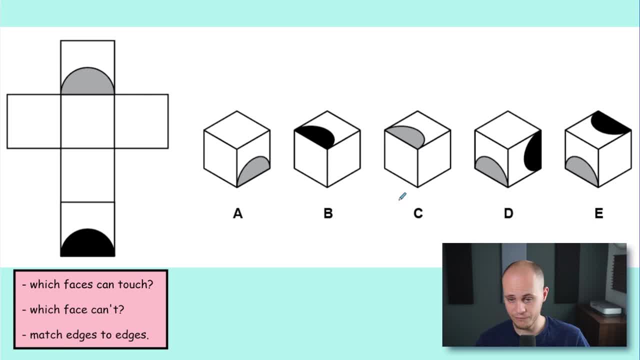 So really nice and simple one. to start with, Use my first tip to solve this one. Think about bringing this square down to the bottom, or, alternatively, bringing this square from the bottom up to the top, which I might do because there's more space. 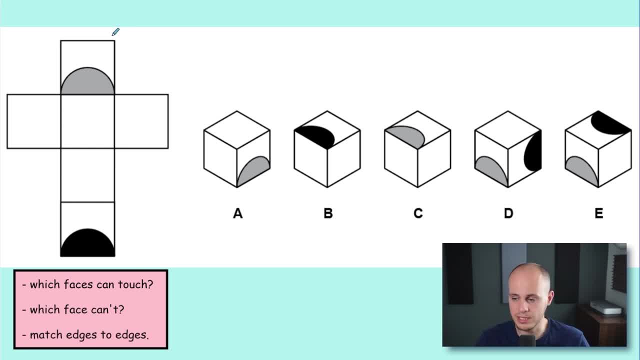 So pause the video and have a go. Which one would be a correct representation of this cube when folded Use deduction. Four of them can't exist, So I'm going to draw the black face of the top here. So I know that I'd have the black semicircle here. 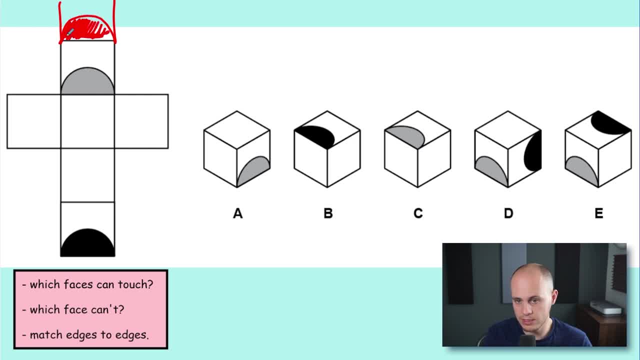 That's kind of cool. It gives me an idea of what they look like. So the semicircles- they don't face each other. In fact they're actually facing the same way, You know. imagine they're pointing this way: 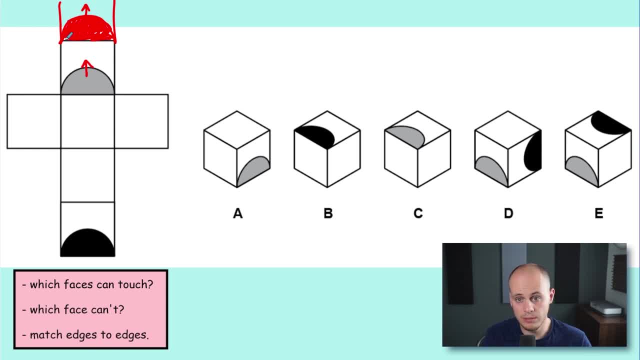 They're both pointing that way, right And below the black one. so if I go to the bottom of the black one, the face directly below it should be the grey one. So, look, I can get rid of B because there's the bottom of the black one. 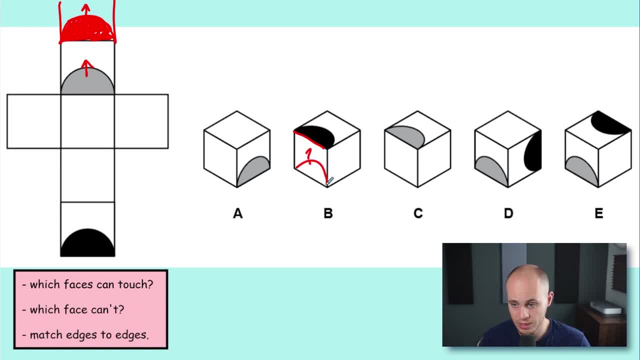 but I see nothing on the face below it, And it should have a grey semicircle. So that's wrong And equally with A, the opposite now applies. Above, the grey semicircle should be the black semicircle, But it's not there. 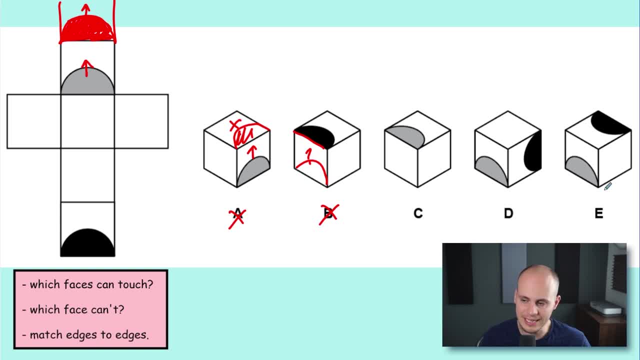 So A can't be right either. Now, looking at D and E, I can quickly get rid of these ones, because look at the way the semicircles are interacting and pointing So that one points that way and that one points this way. That doesn't make sense. 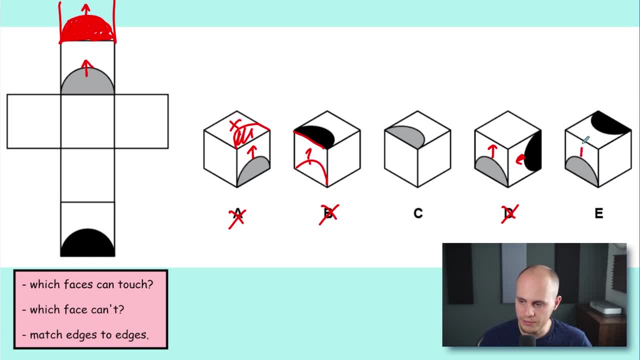 We've agreed. they're both sort of facing the same direction And the same. with E They should be pointing into each other this time, which is completely wrong. So through the power of deduction alone, I know the answer is C and I haven't even thought about it yet. 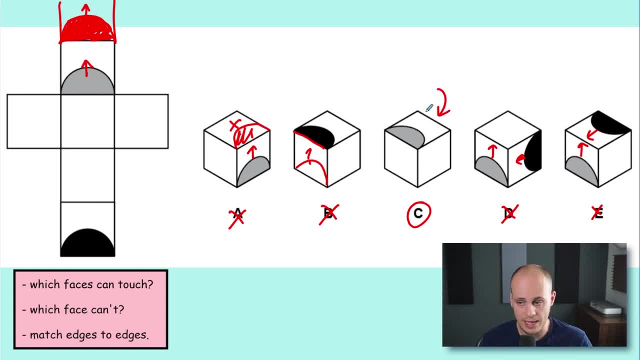 And I can check it, because, actually, do you know what? Even though we can't see the black face, it would be under here, wouldn't it? It does make sense that everything else is blank. There is nothing below the grey semicircle. 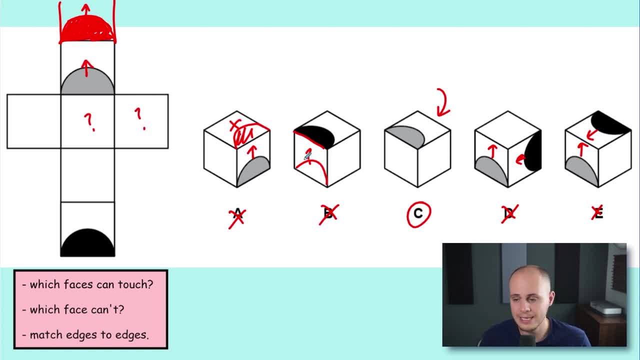 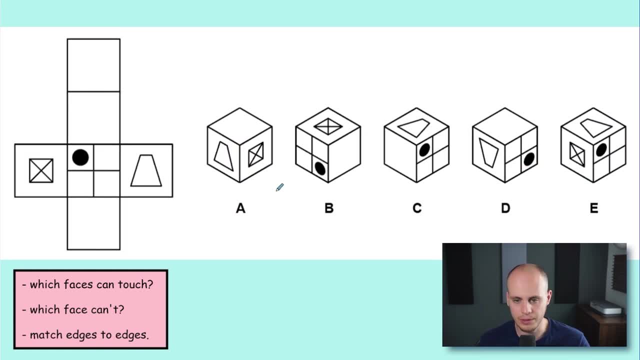 and there would be nothing to the side of it which would be this one. So it completely makes sense that C is the answer. This brings me on to my final trick, which I'll show you at the end of the next question, because it would be easier to do that for you. 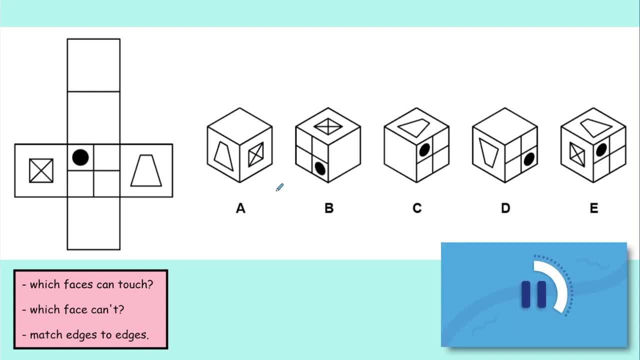 Anyway, have a go at this one. Let's use our rule of opposites to get rid of some answers this time. So I know that this face and this face are opposite. They cannot be next to each other like in A. A is wrong. for that reason, 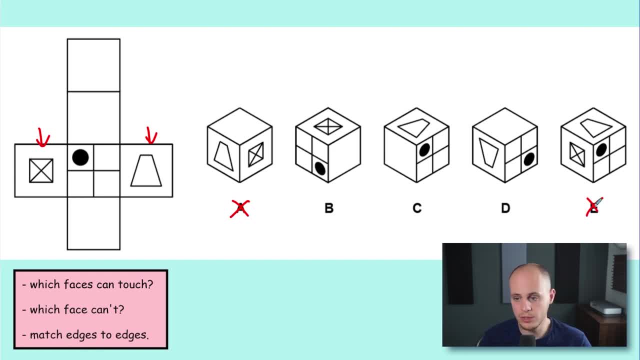 Does it happen anywhere else? It does. It happens in E as well. So we've got rid of two answers just from the opposites rule. Now let's use a positional piece of awareness. So I notice that that dot obviously isn't perfectly in the centre. 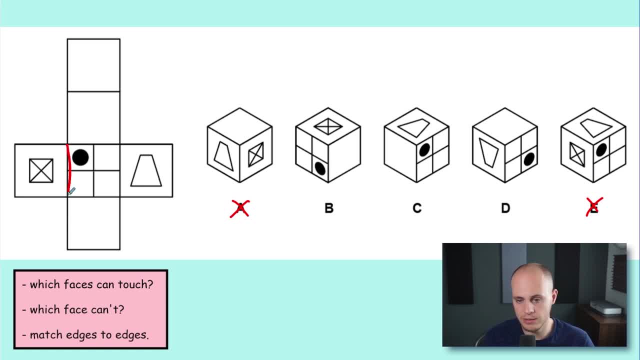 It's more on the side that goes right next to the face, with the cross in it. So I know that the dot should be really close to the cross, not in one of these positions, which would be further away. And equally in the same thought, I know that the dot 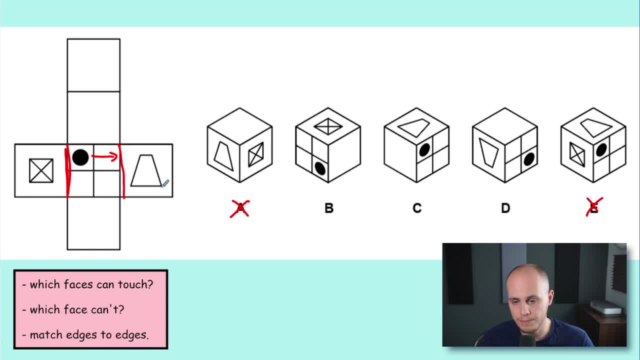 is much further away from the face with the trapezium on it. So let's have a look. B must be wrong because, look, the dot is far away from the square with the cross in it, whereas quite clearly I can see here it's very close. 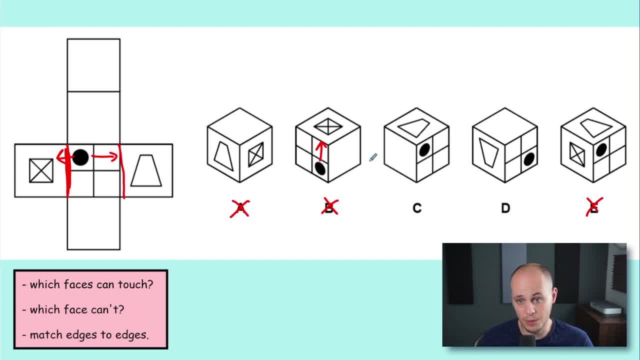 So that can't be right. And the same applies to C, but the opposite way around. In C I can see that the black dot is really close to the trapezium, but quite clearly it should have a blank square gap between them. So that can't be right either. 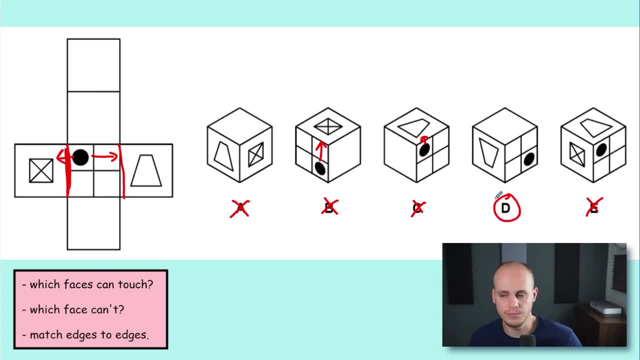 Which leaves me with one answer. Once again, I've solved it with deduction and let's just check: it does make sense? It does, because I've got the appropriate gap now between the dot and the trapezium, like we expect to see. So, as you can see, deduction is coming in very, very handy. 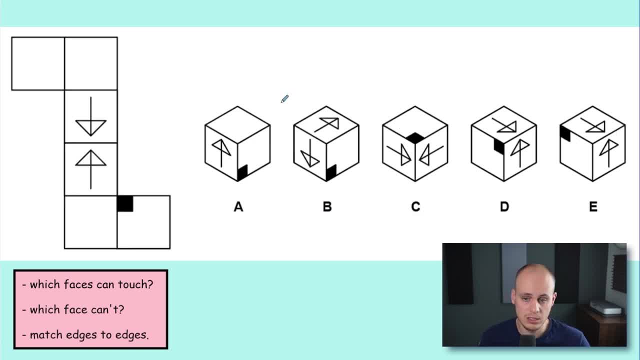 here and we use the rule of opposites to help us solve this one. So you've got next one, and this is the one where I will explain my third and final trick for you, once we go through it together. okay, So have a go. 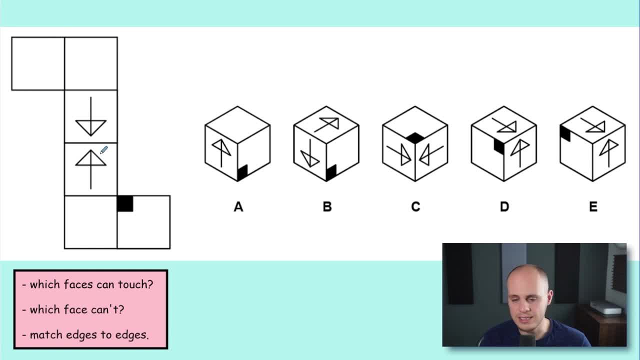 So, first thing that's positional, really handy here with arrows because they're very easy to interpret. The arrows are quite clearly pointing towards each other. They are in faces that are next to each other and they're pointing towards each other, So I can get rid of A 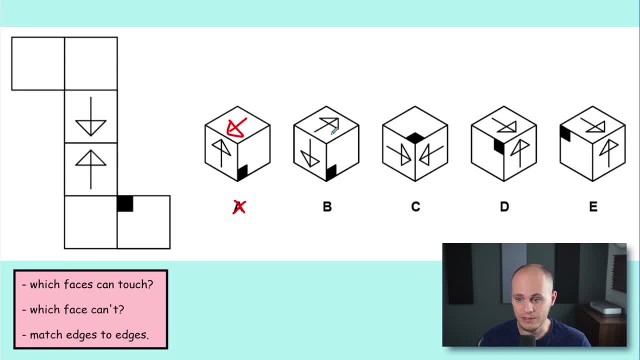 because the other arrow should be there. It's not. I can get rid of B because they're quite clearly pointing the wrong way. C, D and E are all okay regarding the arrow, So the only thing that I can use now to determine which one's right is this square. 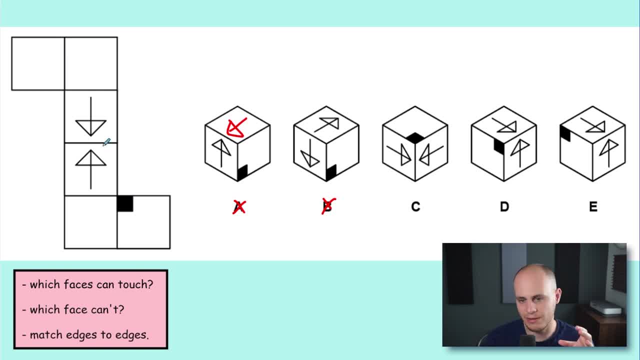 Now you might notice that the square looks like it's nowhere near these arrows, but of course, when things get folded, faces start to touch, For example, this edge and this edge. so any edges that are at a right angle, like this, when folded, they 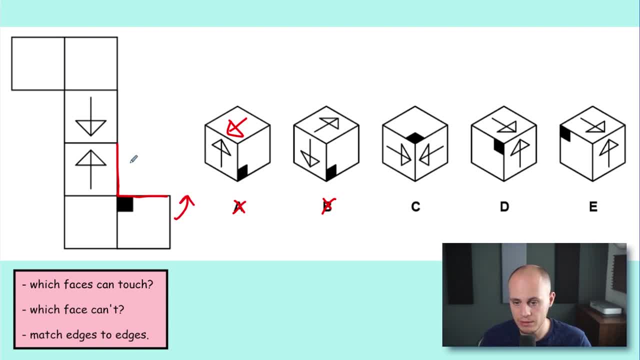 will actually touch, okay, Because this will fold kind of down and this will also fold down and those two edges will end up merging. And what we can do with that knowledge is we can actually draw any of these sort of side faces that are poking off. 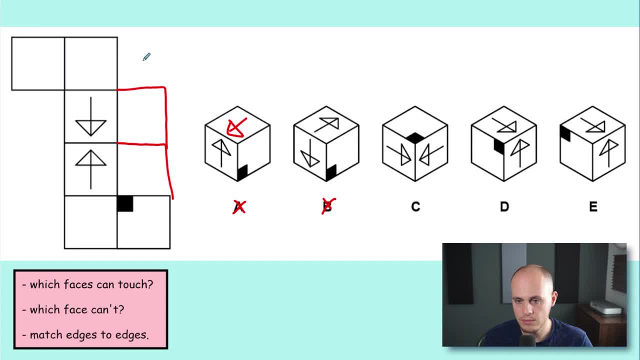 We can actually draw them in any position, up the edge of this that we want to, And all we have to do to draw them in the new position is: we don't just copy them, They don't just translate up, They actually rotate 90 degrees. 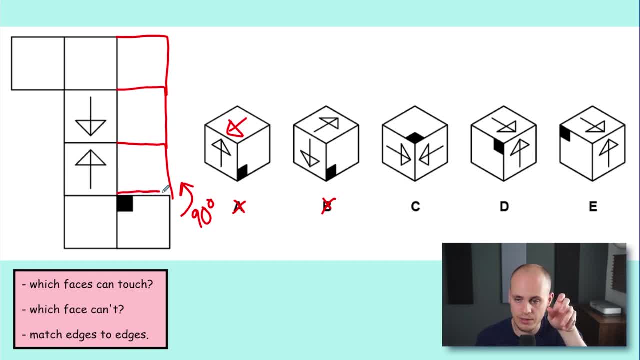 each time. Imagine you're picking it up and kind of rolling it over so that this side kind of closes in into this side Right. So it's currently the square's currently in this corner, but if I roll this around, my square would then be here. 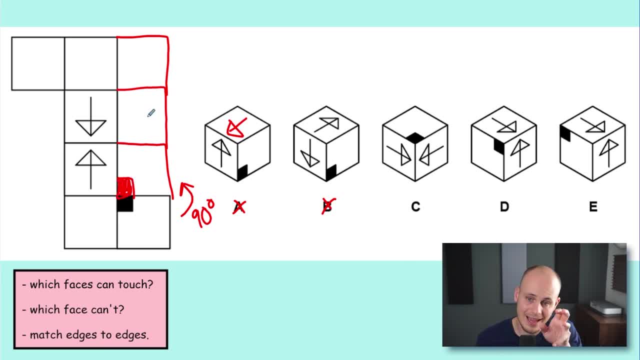 rather than here. And if I was to roll it again and I wanted to move it up to the next one, the square would then be here, If I was thinking about its relationship with this face And if, just for good measure, if I wanted. 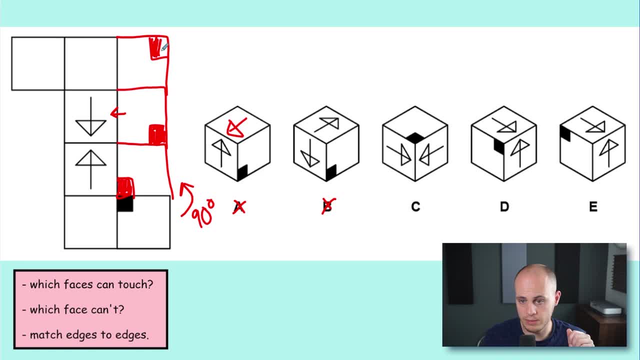 to move it up again. the way it'd react with this top bit is the square would then be there. So if you want to move one of the outside faces so that you can more easily visualize what it would look like next to a different face, then you just have. 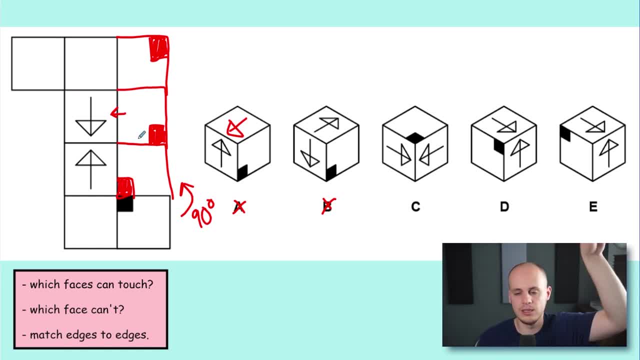 to rotate it as you go. Imagine you're rolling it up up the side of that shape. So how does this help us? Well, look at C and D. C and D both have this square right smack bang in the middle of where. 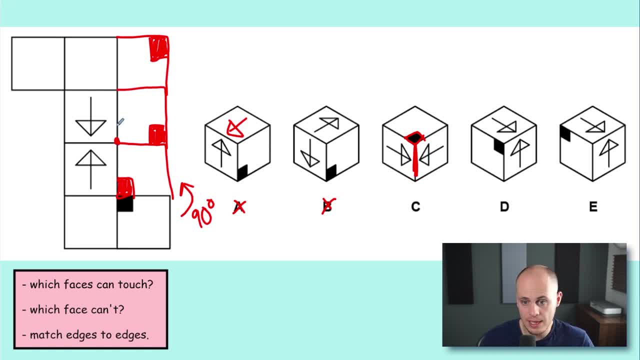 the arrows meet, Which I would represent as being here, Either there or there, And I've just proved that it is neither in neither of those positions. Okay, So it can't be C and it can't be D. Another way to think about it would be: 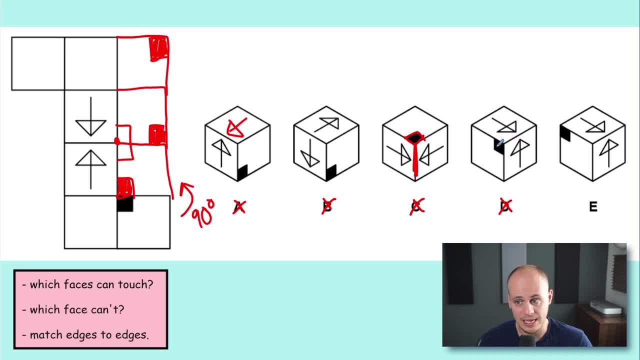 C and D are technically identical. if you think about it, C is the same as D. I could just move that cube around And we can't have two answers So clearly that by definition of C and D being the same means they can't be right Otherwise. 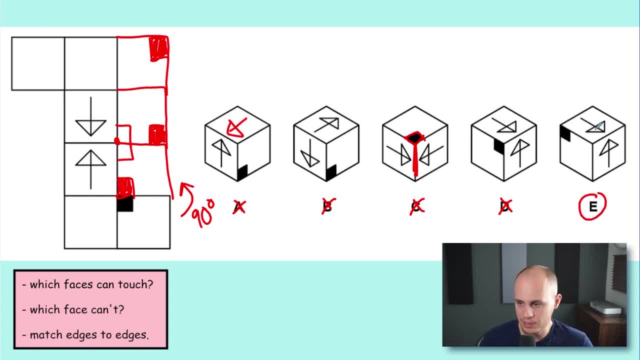 we'd have two answers. So leaving E is the last one, And it makes sense because, look, we've got the square at the kind of back end of the arrow, Which makes sense because, look at the back end of the arrow, that's where I drew it when I 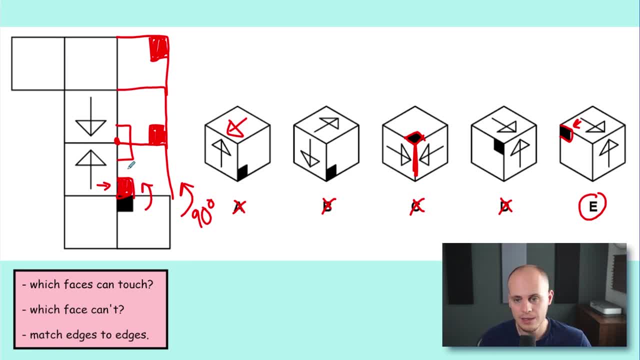 rotated this around into a new position. That's my third trick. It's much harder to visualize, But you just need to remember that if you want to move one of the outside squares, you can just roll it up the side, rotating it 90 degrees each time and drawing it. 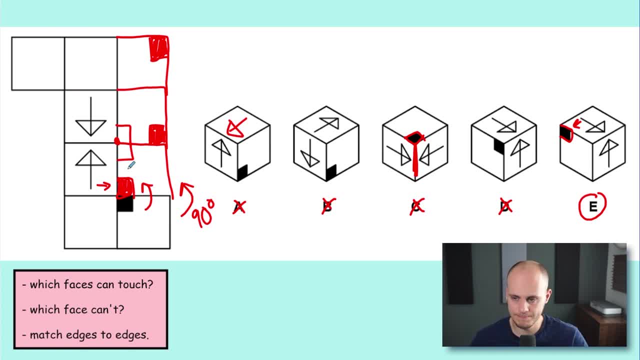 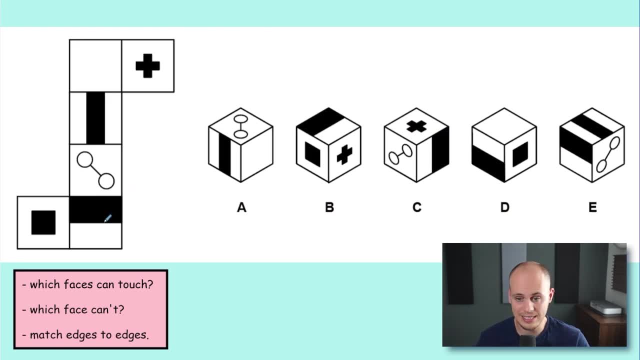 in its new position to see how it relates to a different face. Okay, Tricky right, So let's put all of that together. Here's a really hard question. You can use things when you've got lots of faces, use opposites. 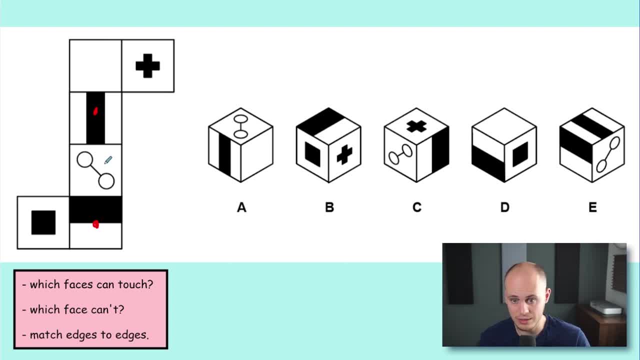 So you know that this one and this one are opposite. right, You know they're opposite. You know that this one and this one are opposite. You also know that this one and this one are opposite. So you've got tons of opposites to play with here. 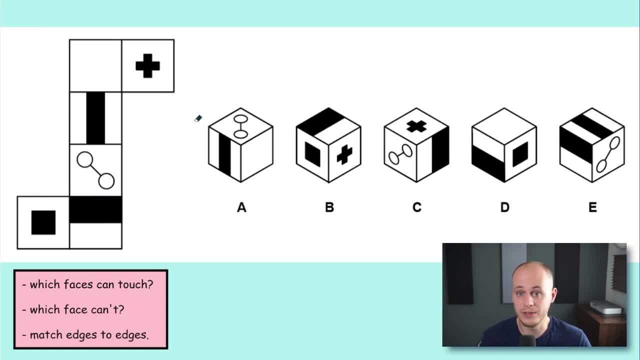 and you can use that to your advantage. when you solve this one Off, you go Right. well, let's do exactly that, okay, I know, firstly look at A. I know that this two circle with a line in between it is opposite the only blank side, that's in. 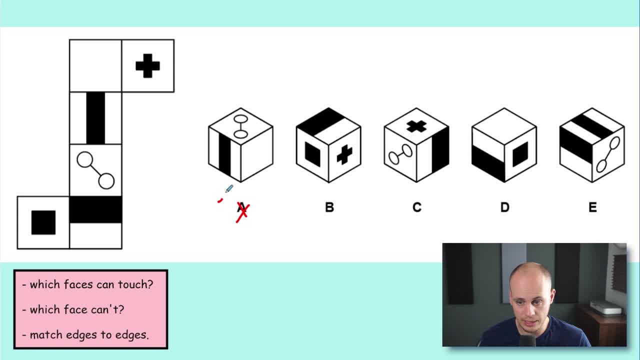 this cube And quite clearly in A it's next to it. So that's wrong. The blank side should have been opposite. Moving on, Does it happen again? It does look. I know that this square and this cross here I. 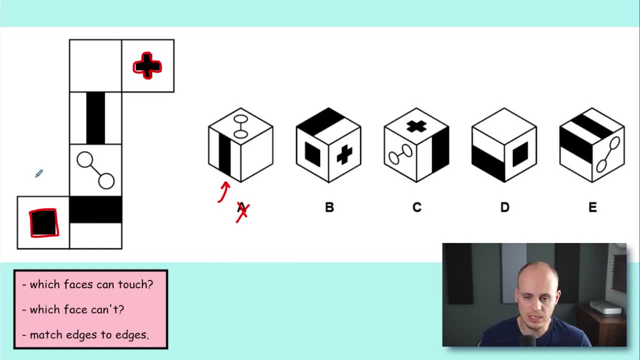 know that they are opposite as well, Because they are the two pieces on the end. I could rotate this all the way up here and have it drawn up here, just to prove that it would be the opposite. okay, And it would actually look exactly the same. 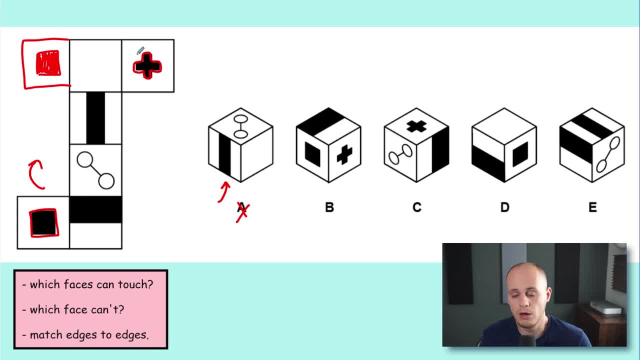 because it has complete rotational symmetry. So I know that these two are opposite. So B doesn't work either, because they're right there and there. okay, Let's look at C. Let me get rid of my drawings for a minute so I don't complicate this. 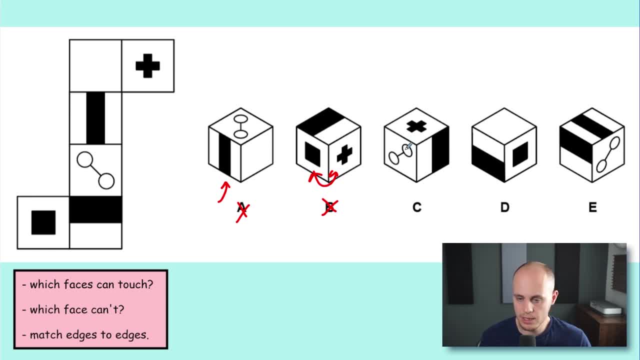 Okay on C: Well, okay. so if we look at this, yes, this is interesting. It's a positional relationship now between these two faces. So I notice that the two circles, when they meet with that face, that's got half black, half white. they actually 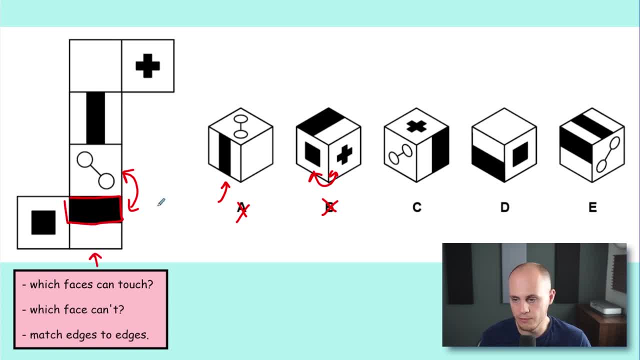 touch the side that's half black. They don't touch this side that's half white. So C can't be right, because the two circles with the line in between are touching the face with the white half. So that's wrong. That's the wrong way around. So we've got D and E. 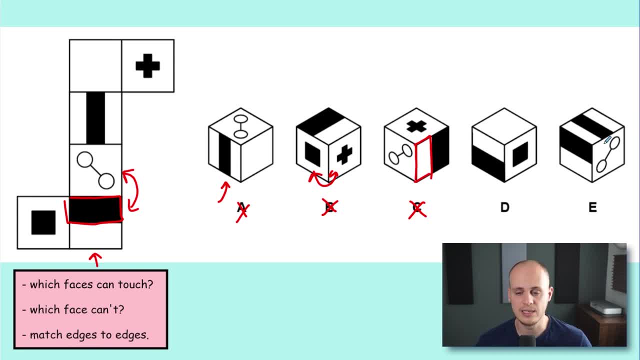 At this point. I quite often look at both of them just to see if there's a quick fix to help me here. Okay, Is there anything we can do really quickly? Well, I guess E is something we can use, because look the way the two circles react with this face. 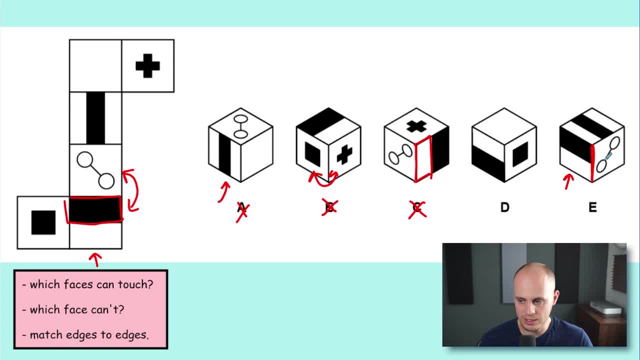 again here. this face is completely the wrong way around because it's now touching a bit of black and a bit of white. It should be split this way, and this bit should be black and this piece should be white. So E is also wrong because of the way it interacted with. 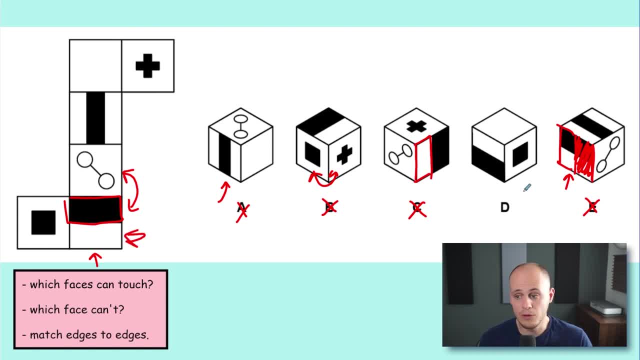 this bottom face. here D must therefore be the correct answer, and we can also prove it, because we know that to the side of the black and white piece is this face with a square in it, which is exactly what's happening here To the side. 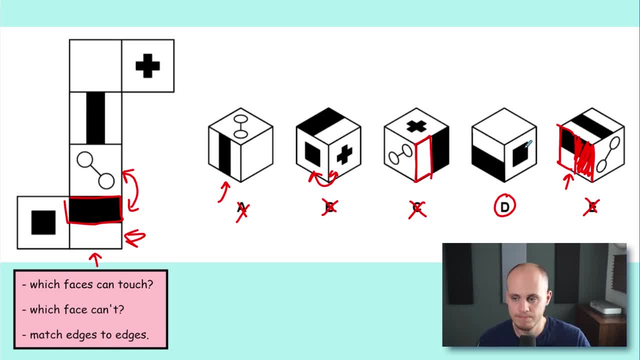 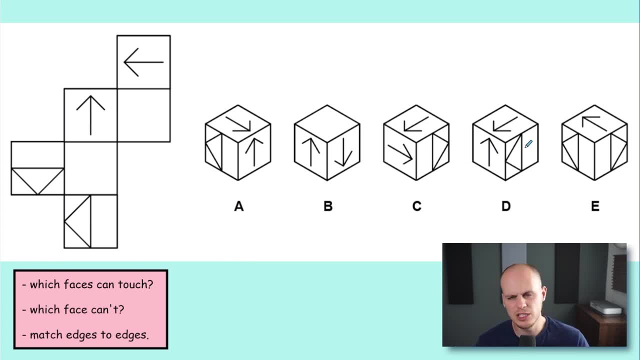 of this is the face with a square in it Makes sense. Last question for you, Nice and horrible one to finish up on, but it's worth having a go. Think again about the positions of things. Maybe you can roll this around. Okay, To notice that this arrow. 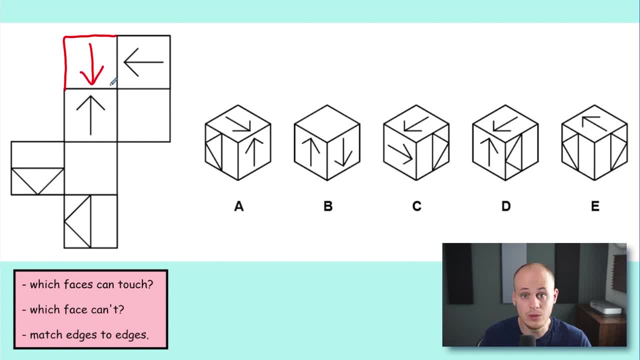 would actually be when folded. it'd actually be pointing towards this one, Right? Can you use the same logic down here and we can use some deduction? Have a go. So I thought it was really interesting. Obviously, this happens. So those two red edges. 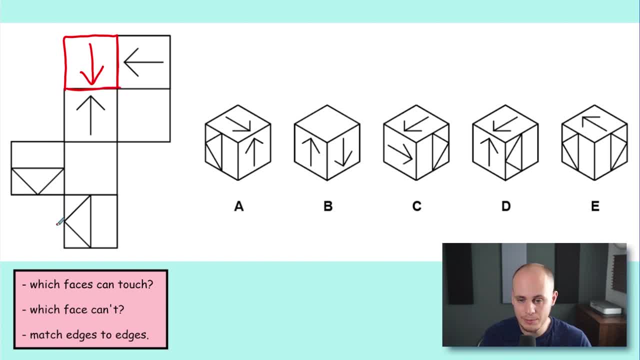 will touch and the arrows will actually look like they're pointing towards each other. The same would happen down here. If I roll this edge, this face around- Okay, I'd actually get this, So the points would even be touching in this case. 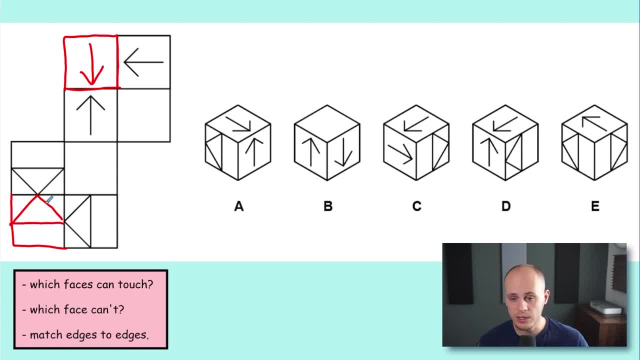 So I can use this to get rid of four answers and just solve this purely on deduction, Not really imagine folding it in my head, Okay, So anywhere where the two arrows aren't pointing at each other, get rid of it. So B's gone. 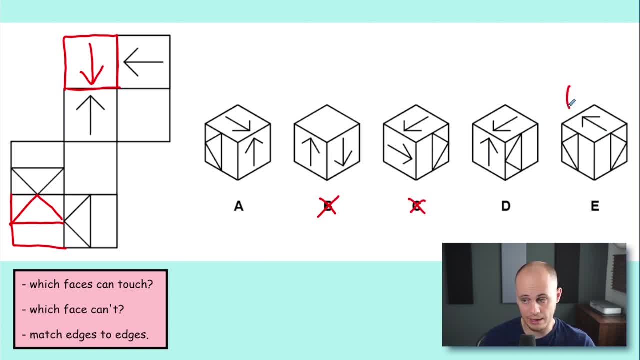 and C's gone. I don't know about E, because there could be an arrow behind there, and that's okay. Now, anything where these two triangles aren't directly pointing towards each other we can get rid of. So I can get rid of E, Unfortunately. 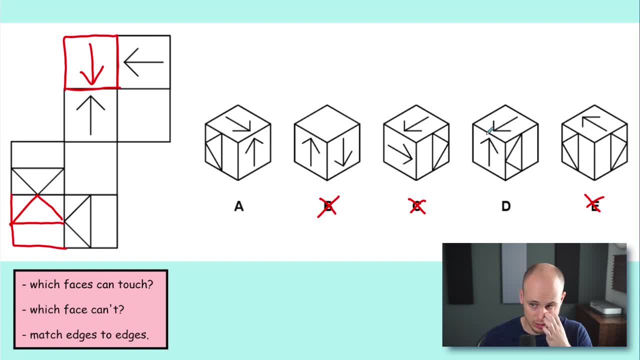 with D and A. in fact, I can get rid of D as well, because look, it should be here And it's not. There's an arrow there, So we've already solved it Done. I was about to say with A. we don't know if it's that side. 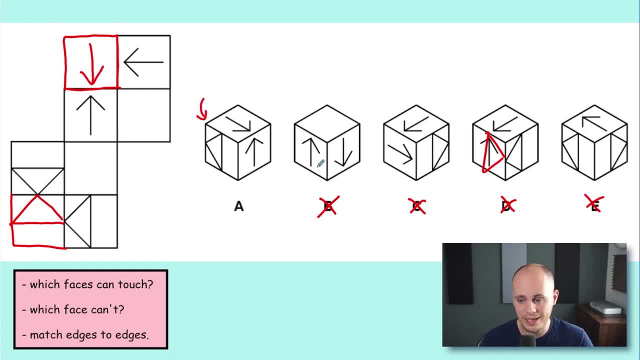 or not. Well, now we do, because we know it's the right answer. We got rid of everything else with deduction A is the answer. So, even these horrible questions, by using those three tips that I showed you, I'll whisper them again now for you before: 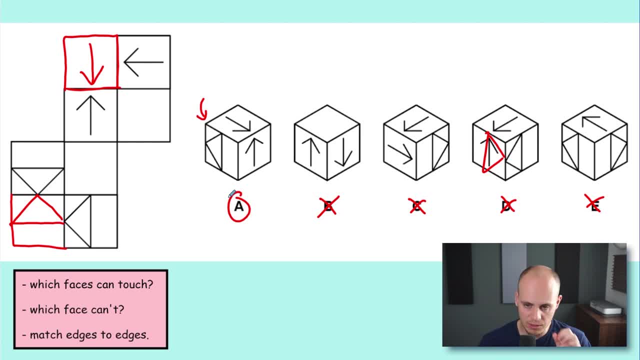 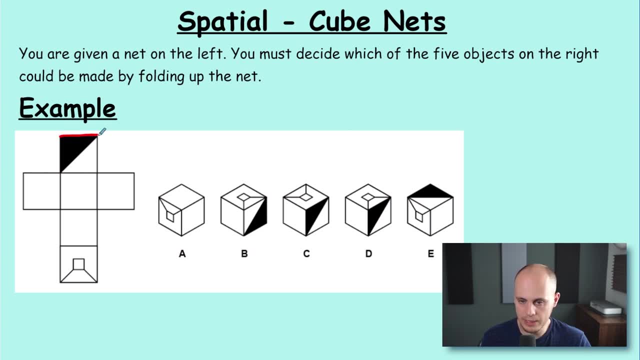 I go. you can solve anything with deductions. Those three things were as follows. Let's go right back to the start. First thing is just knowing that we can draw pieces in new positions. For example, we can take the top piece and put it. 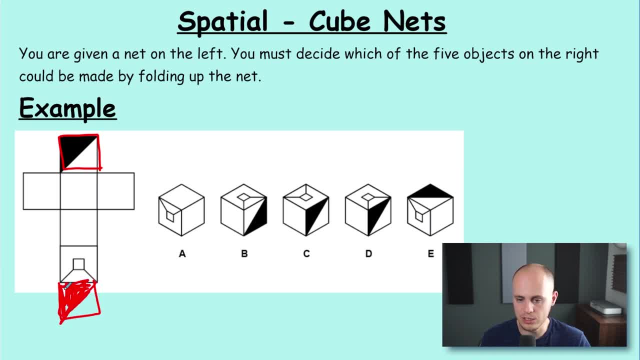 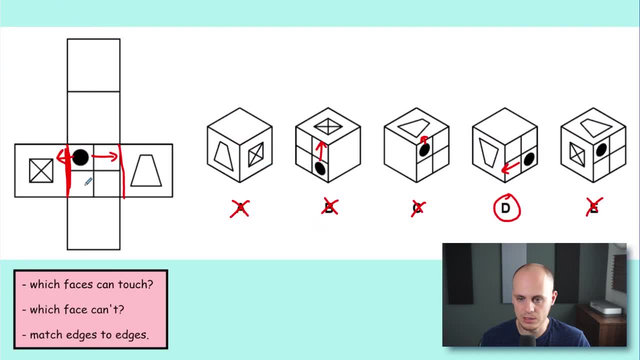 at the bottom so that we can more easily see how these two correspond to each other. That was tip number one. taking that, Tip number two was understanding opposites. So if I go to one of the later questions where it was really helpful, like in this one, it was just: 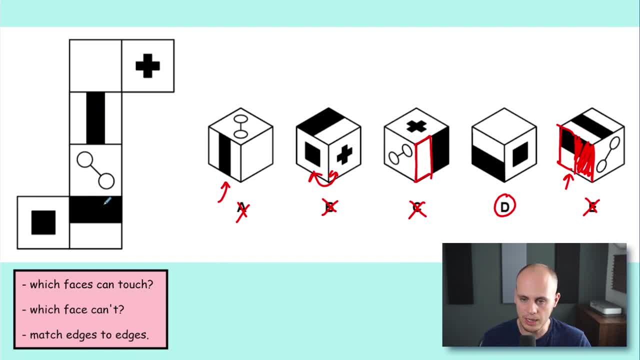 knowing that things that are two apart down the main spine, so this one and this one are opposite, that one and that one are opposite, and also knowing that the two pieces that come off the edge, when they're folded down, they would become the ends of the cube. 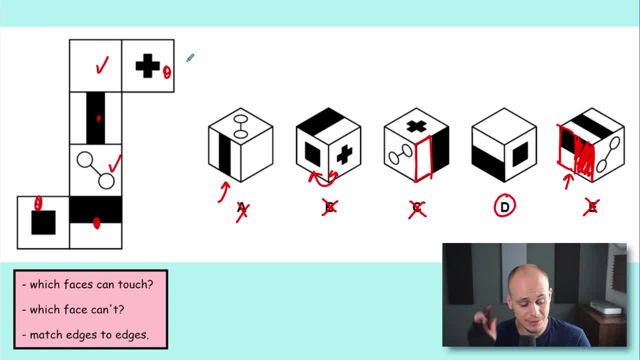 and that they would also be opposites. That's opposite. So that's my second tip, And the final one was the slightly harder one. It was just knowing that if you want to take one of these end pieces, like in the last question, 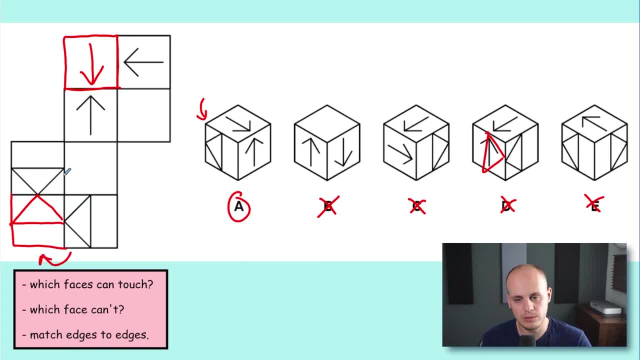 if you want to imagine it in a new position of how it would relate to another face, you can rotate them 90 degrees around. So as long as you're rotating it 90 degrees, you can draw it in a different way. It would still be correct. 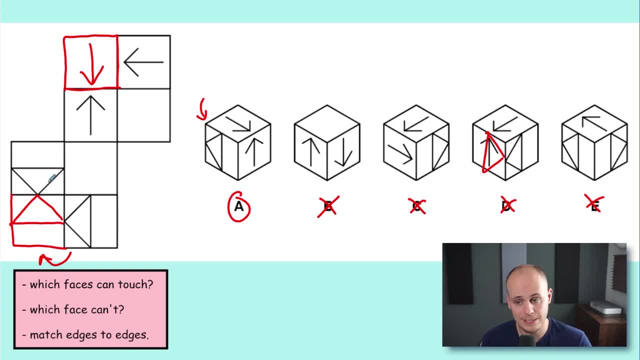 it would just be where that face was in relation to another face, And that's it.